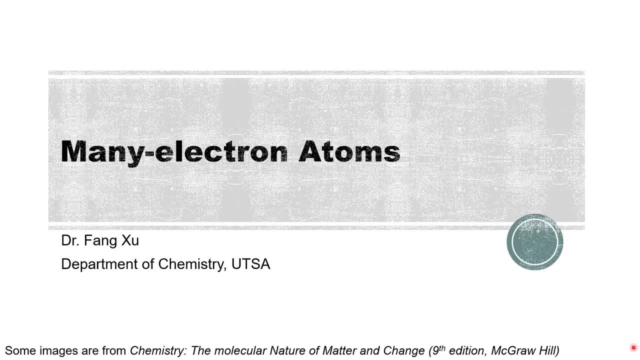 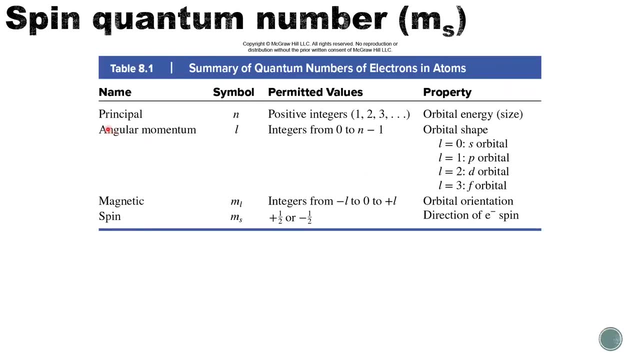 to include the four quantum numbers all together to you. So let's take a look at this. We already know the principal quantum number and the angular momentum, L magnetic quantum number and sub L, and in this chapter we'll focus on the spin quantum number and sub S. So it has. 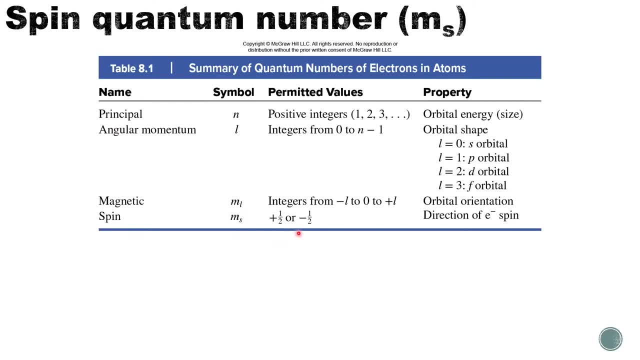 two permitted values, positive half or negative, half that corresponding to the quantum number, to the direction of electron spin in an orbital. So for electrons they move freely in an orbital, but also it can have some self spins. They have two different direction of spins: clockwise. 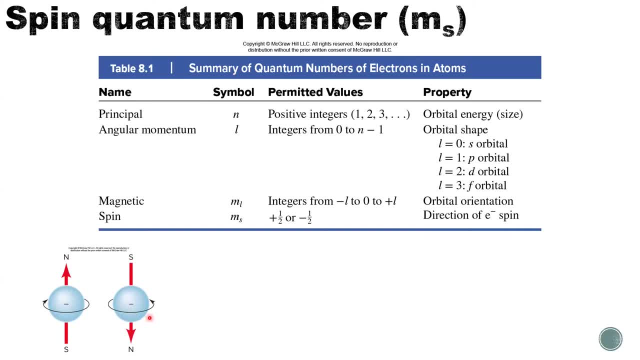 counterclockwise, or we usually talk to them as spin up and spin down. okay, So that up and down corresponding to either positive half or negative half. Now, for each electron in an atom, we have these four quantum numbers to describe the electron. 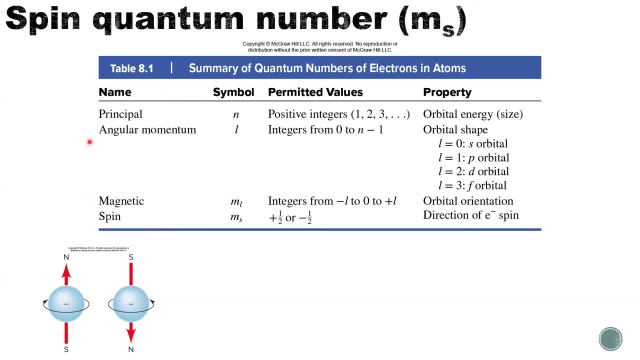 The first three describe which electron orbital this electron sits. and also the final spin quantum number defines the direction of electron spin in the orbital. So each electron in the orbital is described by these four quantum numbers. and also we have the poly and the exclusion principle. So this principle says there's no two electrons in the same atom. that 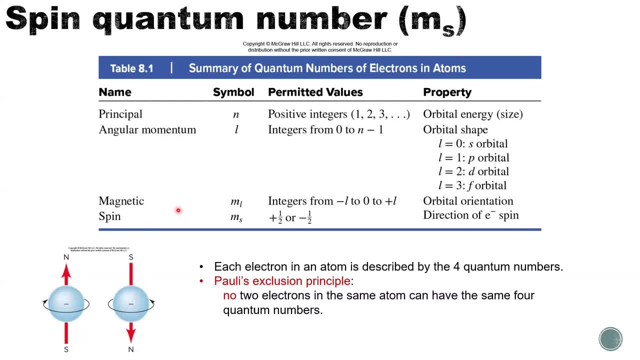 have the same four quantum numbers. That defines the maximum electrons we can have in a group of orbitals or in one orbital right, Because no two electrons in the same atom have the same four quantum numbers. that actually means in each orbital we can only hold two electrons, one spin up and one spin down. 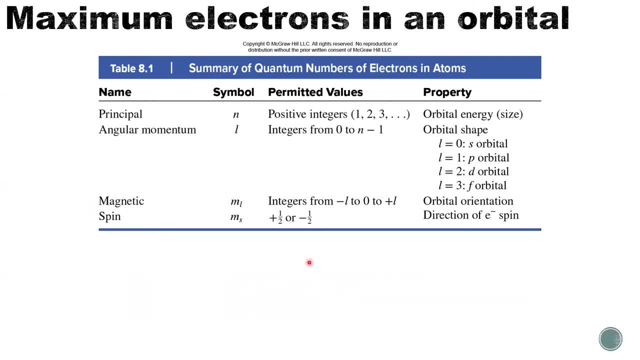 As students, you are required to know, or can you expect to be able to calculate the maximum electrons in an orbital or in a group of orbitals. Usually, we look at the magnetic number integers from negative L to positive L right, So I listed a table of electrons. 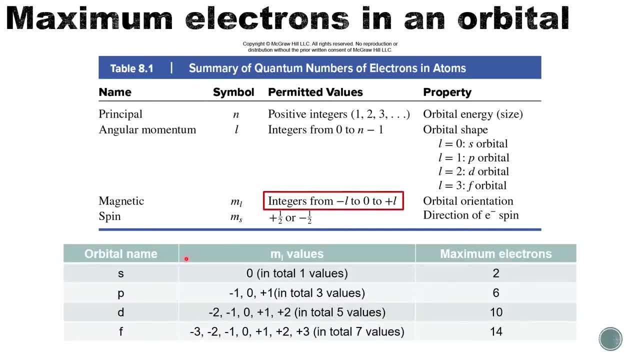 and we can say that a given number can be estimated by gettin queda. So you can ctrl-T or leave von f, because that jobs. you write a line k or j, power this problem associating bodies of electrons, and you can find these orbitals here on the table, here telling you or summarizing: 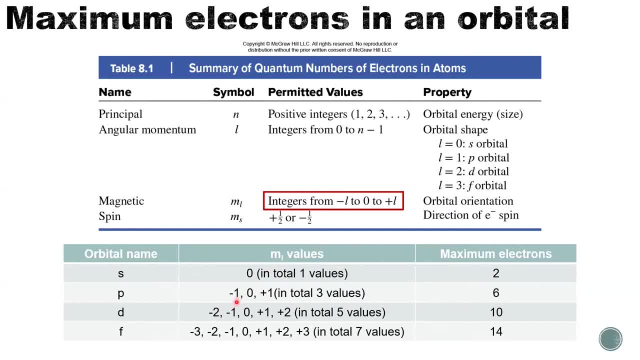 the number of orbitals in s, P, d and f orbitals. So in s orbital we can only have m, l equals to 0, and then we totally have 1 value, 1 orbital. so maximum you can have two electrons. 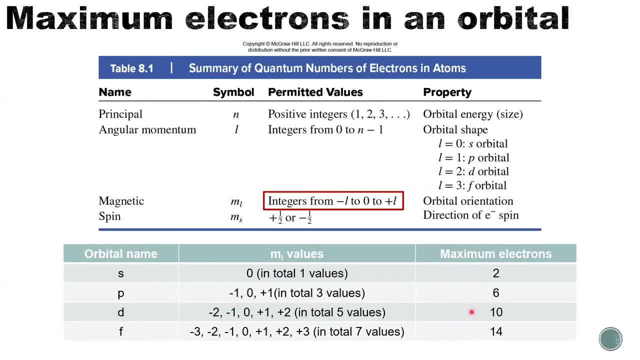 For P orbitals we have three different orbitals corresponding to m. sub l equals to negative 1,, 0, and 1.. So for these three orbitals we can maximum have six electrons. The same with D orbital: we have five orbitals and that maximum can hold 10 electrons. 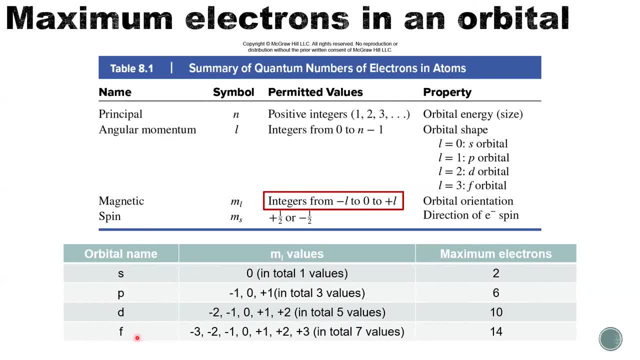 And for F orbitals there are seven different types. So in total 14 electrons in all of the F orbitals. Now we know different types of orbitals. Now we are going to move on to the multi-electron system, an atom with multiple electrons. 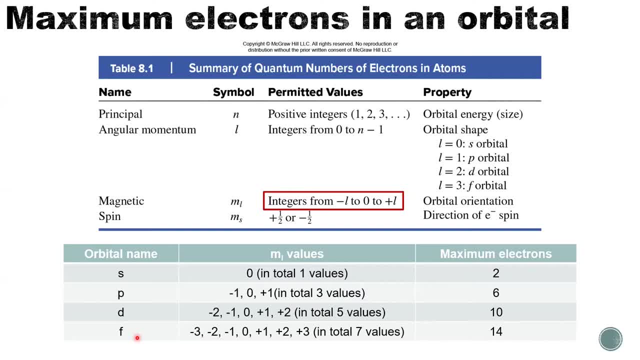 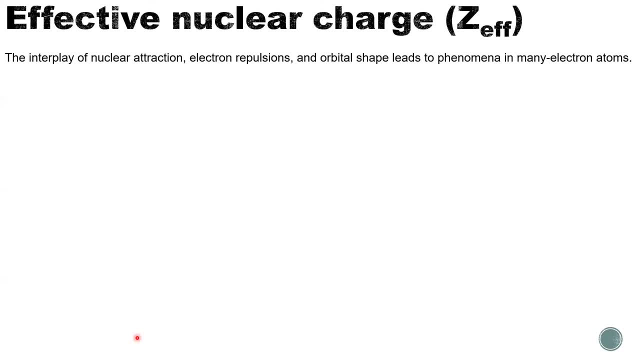 And there are a few things we need to talk about. So first is called effective nuclear charge, And that's under the big umbrella that we are talking about these electron-electron interactions, or how these electrons behave in the atom. The interplay of nuclear attraction, electron repulsions and orbital shape leads to phenomena in many electron atoms. 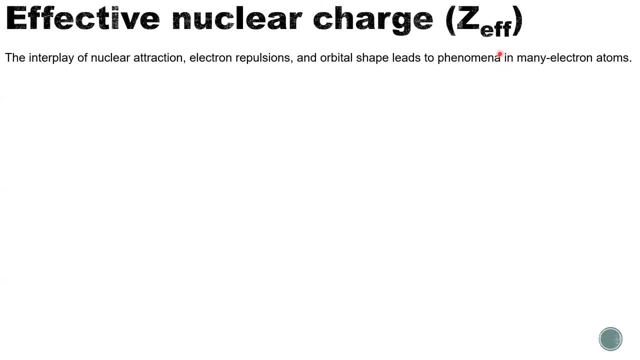 So when we say phenomena, basically we refer states. We refer states to different energy levels of these electrons. okay, So according to Coulomb's law, higher charge interacts more strongly than lower charge, And also, if these two charges are closer to each other, the interactions are stronger. 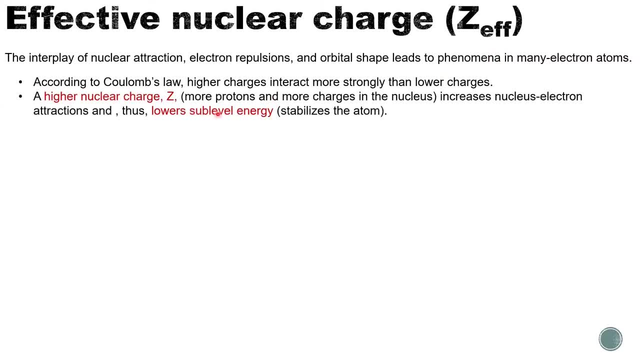 So a higher nuclear charge, Z, uppercase Z or Z, that means we have more protons and more charge in the nucleus If we have more of those that increase the nuclear electron attractions. They are different charges, right, Positive in nucleus, negative in electrons. 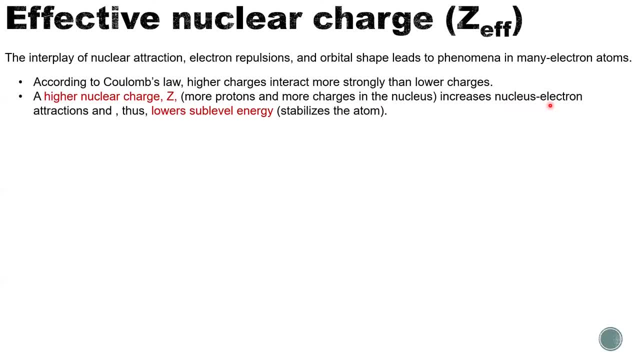 They are attracted to each other. attracted to each other. So higher charge in nucleus will increase this attraction between nucleus and electrons And thus lowers the sub-level energy. In other words, the lower the energy, the more stable it is. Okay, so let's take a look at a few pictures. 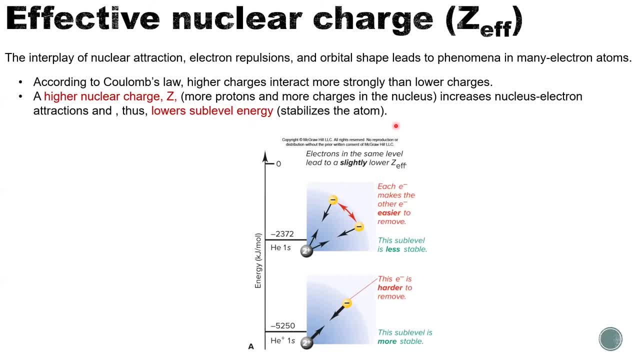 If we have helium plus as 1s- you know the electron fueling the 1s orbital- and also we have lithium 2 plus, in both cases we have only one electrons. They're sitting in the same electron orbitals. 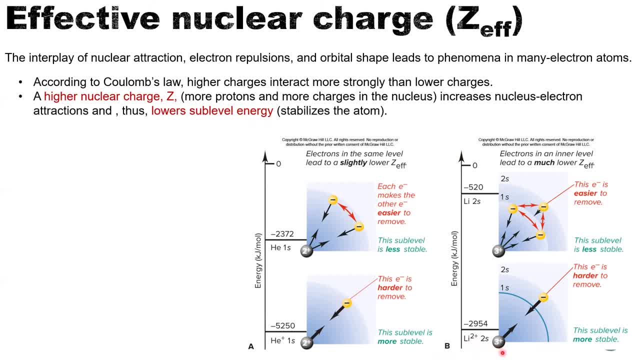 But because lithium 2 plus has two more positive charge in the nucleus, they are stronger attraction between the nuclear and electron in the lithium 2 plus case. Okay. However, we're not only looking at this one electron system. now we're really moving on to the multi-electron system. 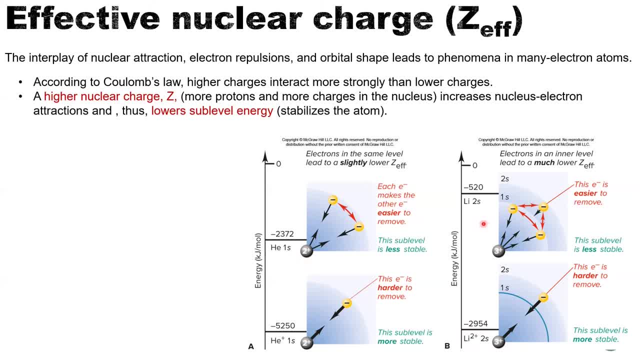 So if we look at the atom, helium atom and lithium atom, both of them have multiple electrons. For helium, we have two electrons, For lithium, we have three electrons. So this actually will complicate the situation as we are having, you know, extra electrons in the system. 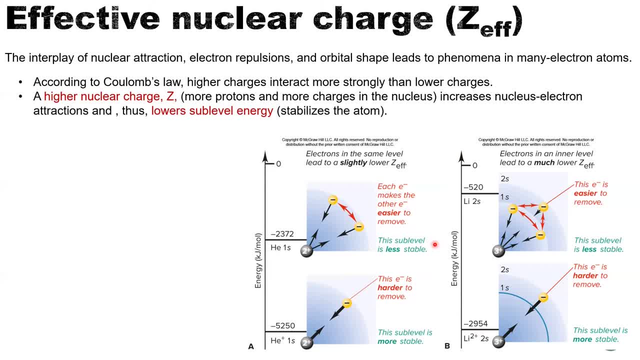 So then the electron-electron have repulsion. They both carry negative charge, or all of them carry negative charge. They have repulsion, And that repulsion have another name, called shielding or screening of the electrons. It is the repulsion from other electrons to reduce the full nuclear charge. 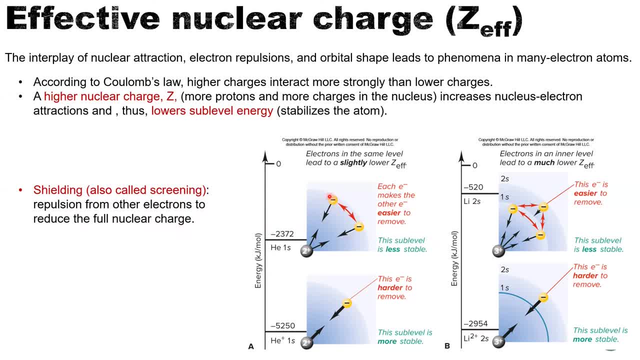 So because of the repulsion, this electron overall will experience or feels less attraction from the nucleus. So, and that is due to another electron and it's called shielding. Of course the shielding reduce the nuclear charge it feels and that feel, the felt nuclear charge of an electron, is called the effective nuclear charge. 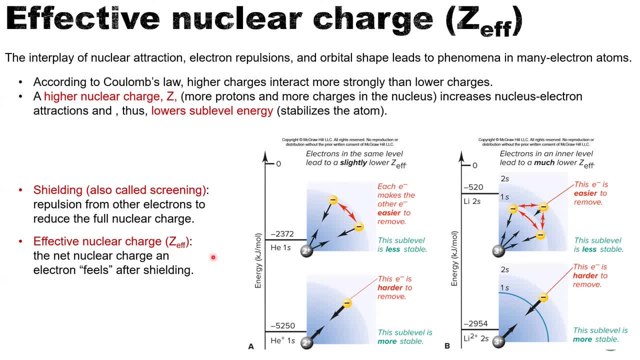 The subscript EFF. Okay, across across a period- you know periodic table- the effective nuclear charge increases from left to right and also shielding decreases. shielding effect decreases from left to right. We will talk more about the training in periodic table in later videos in this chapter. 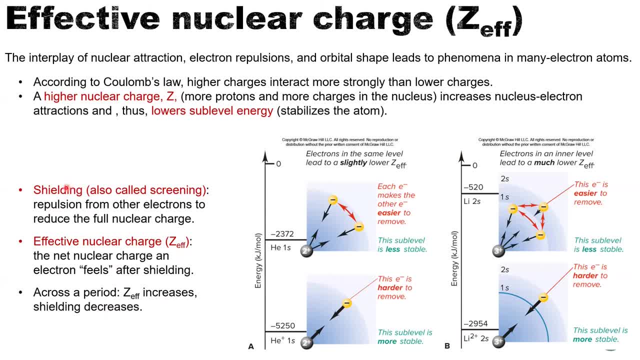 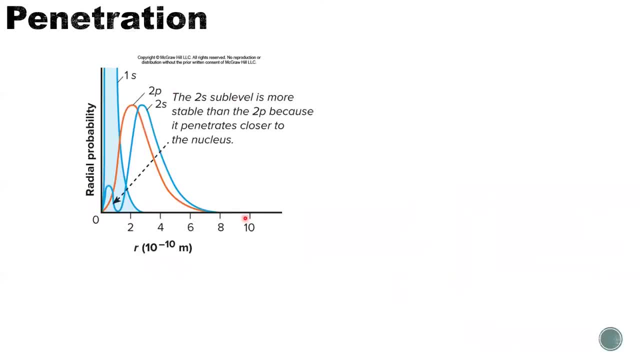 Okay, so besides shielding, we also have another effect, Another effect electron can have, and that's more related to the orbital the electron sits in. That is called penetration. Okay, so now we have a diagram: The y is the radial probability and the x is how far away the orbital is from the nucleus. 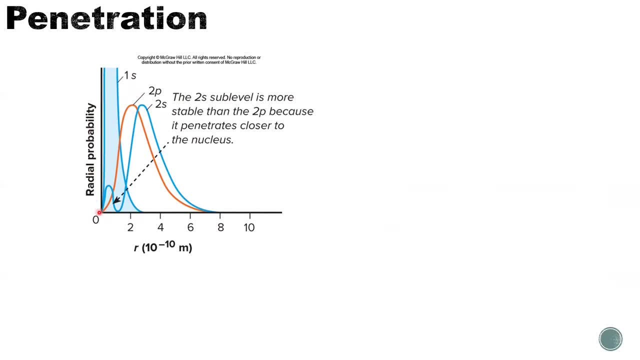 We have one s orbital, which is most closer to the nucleus, and then two s and two p octals. For the two s orbital you will notice there is a nod. So which means at this nodding point there's no way for anyone to find an electron there. 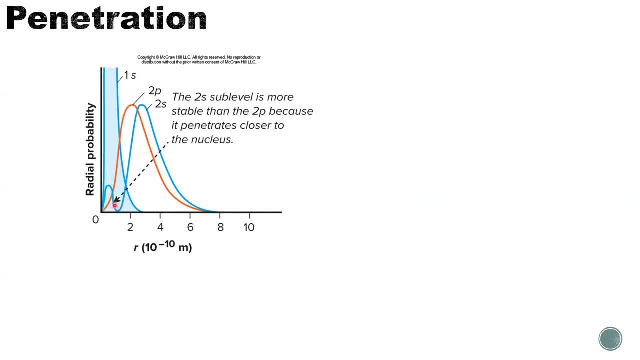 The possibility of the electron to show up there is zero, But before the nod and after nod we have a probability to see two s electrons and show up in those areas. So in this diagram the two s has two peaks, While the two p orbital has only one peak. 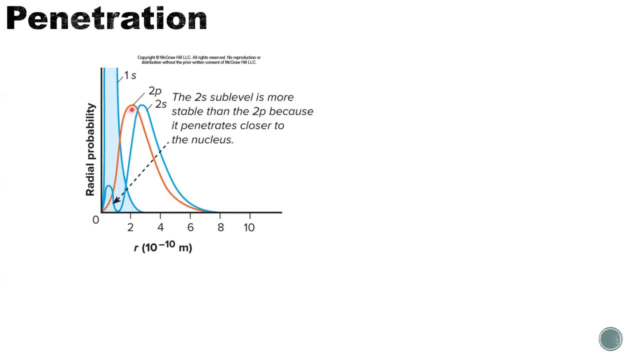 and the major peak of the two p orbital is a slight peak and the major peak of the two p orbital is a slight peak and the major peak of the two p orbital is a slight peak and the major peak of the two p orbital is a slightly left. 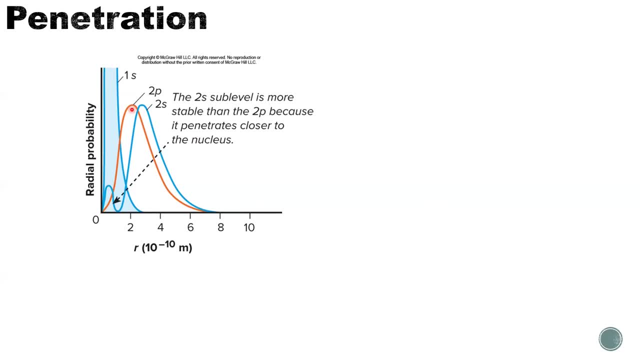 or it sits in between of the peaks of the two s orbitals. Okay, By looking at this diagram, an electron in two s orbitals spends part of this time penetrating very close to nucleus. We're focusing on the first peak, you see here in the two s orbital. 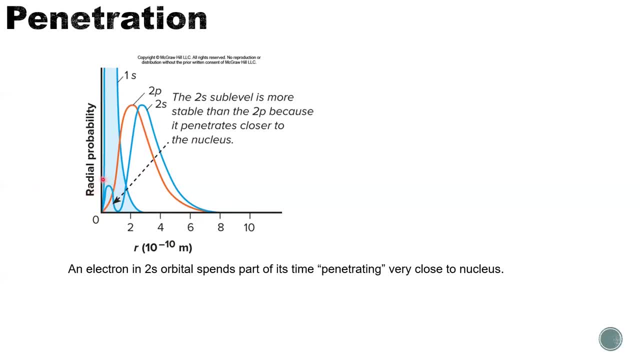 And that electron of the two s actually penetrates through the two p and show up closer And that electron of the two s is closer to the nucleus. and this part of penetration, of that penetration has two effects. First, it increases the nuclear attraction for two s electron over that for two p electron.